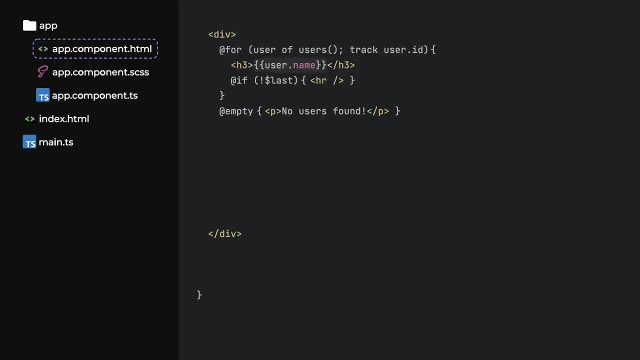 This method is known as the ELS template, which is the new template of the RSS file, added fine-grained signals reactivity and the team decided to make the best of this situation. As a result, we can now use a new built-in control flow which stands out clearly from 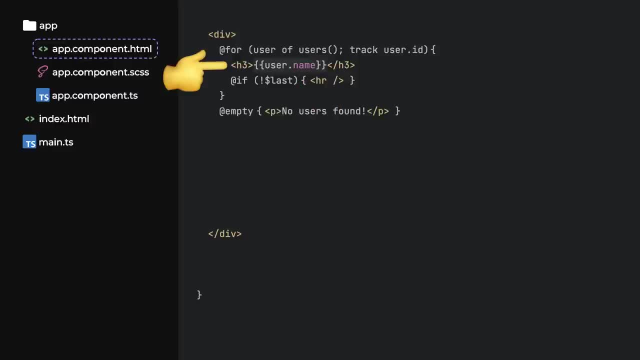 the rendered markup. We are iterating through the list of users and rendering a name in the DOM. Note that you are forced to use the track statement so that Angular can optimize them. updates when the underlying list changes, Also inside the for construct. 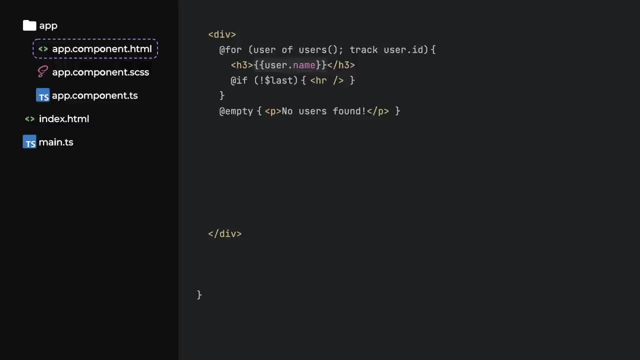 you'll have access to helper variables like index or last, Besides the usual for's and if's, Angular 17 introduces the defer construct, which gives you full control over lazy loading parts of your application. This is a big step forward towards better performance, but 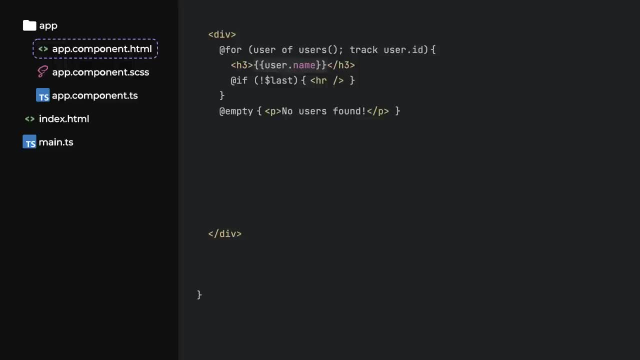 before looking at it in more detail, let's allow users to push data in our list. Back in the component file, I am adding a boolean signal based on which, in the template, I am conditionally rendering a toggle button and a form. This gives us the chance to use one of the 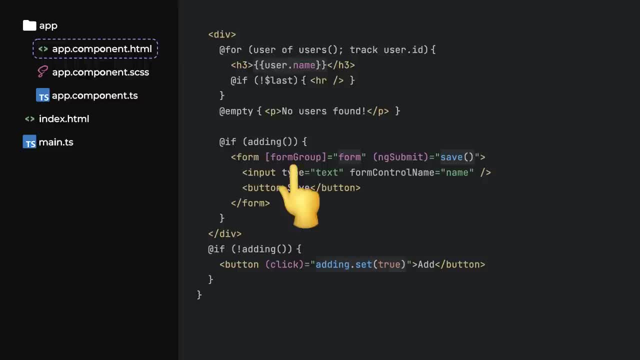 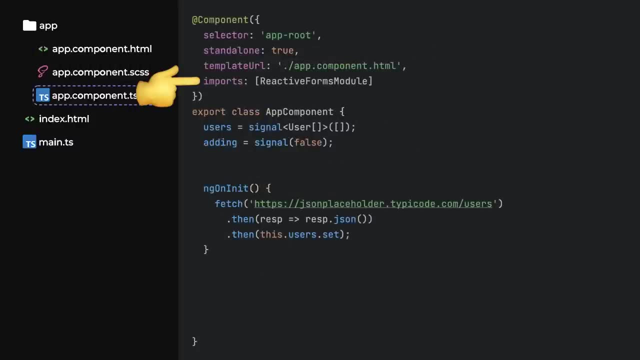 most powerful Angular features: Reactive forms. Let's bind this form to a value in the component and define a handler for the submit event Back in the TS file. we first need to import the reactive form, which is the one that will be used for this task. 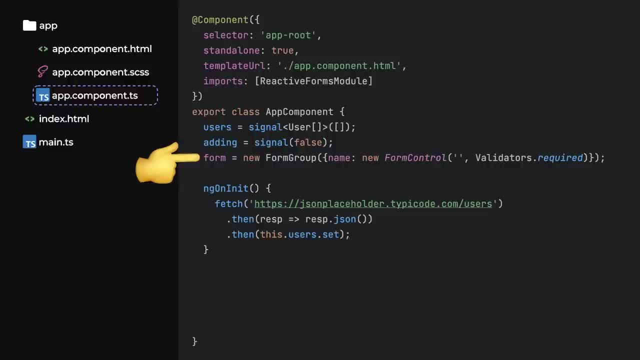 Then let's define a form group with a required form control. Finally, in the save method, when the form is submitted, we are pushing the new value in the user signal. Now let's discuss the rendering strategies aimed to improve the performance of 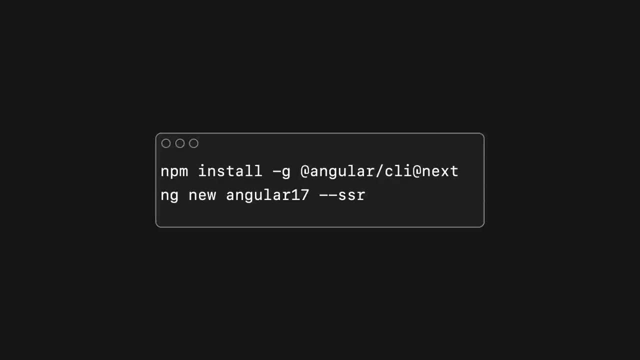 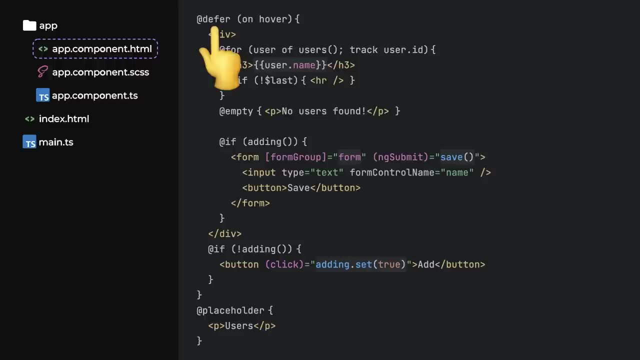 your app. First, it is worth mentioning that, starting with v17,, you can create a SSR-enabled app with this simple command. The real power, however, is brought by the new defer block. With this one, you can lazy load parts of your application for better initial user experience. 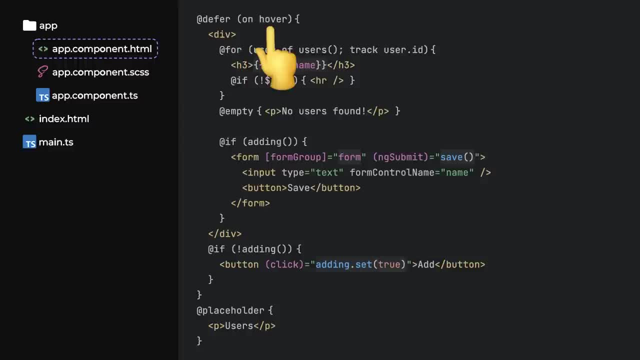 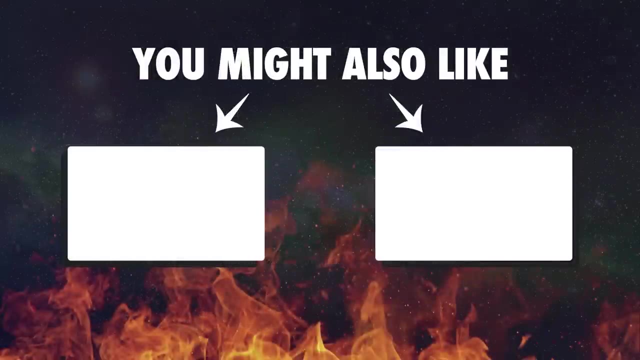 and overall improved performance. There are a handful of triggers which will cause defer sections to be rendered, and a block can be paired with a placeholder to display some dummy content until the real data is rendered, While Angular is making big steps forward, I get it might not be your cup of tea. If that's the case, here are some more recent UI frameworks. 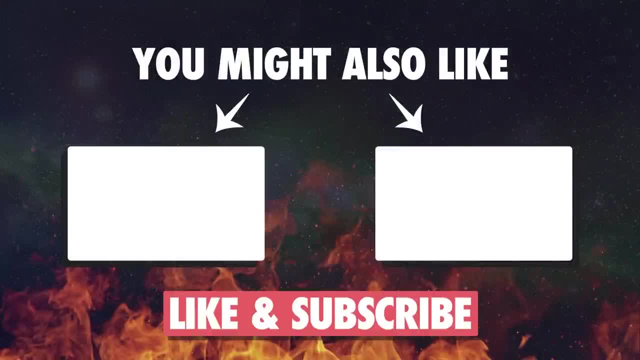 which are making big waves in the industry. Until next time, thank you for watching.